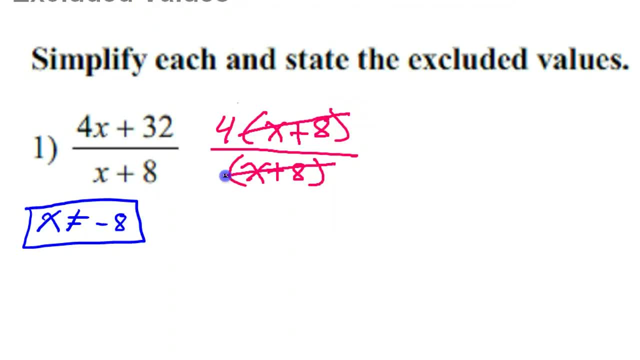 So they will cancel out because they are the same factor. Alright, so the simplified version of this is simply: four, Okay, four, Four. So let's put this all together into one answer, and then there you go. Alright, so this is the simplified answer with the excluded values. 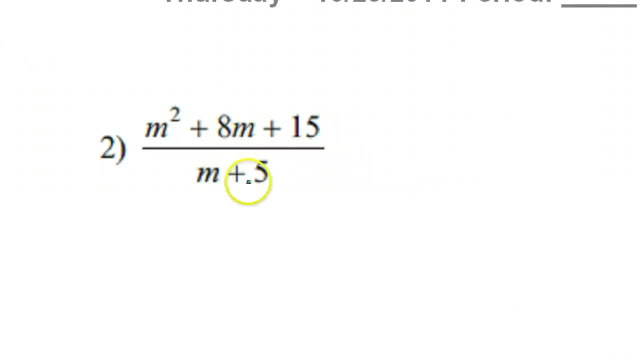 Let's take a look at number two. Alright, again, I can get the excluded values by noticing that the denominator cannot equal zero. Subtracting five from both sides means that m cannot be negative, So that is my excluded value, right there. 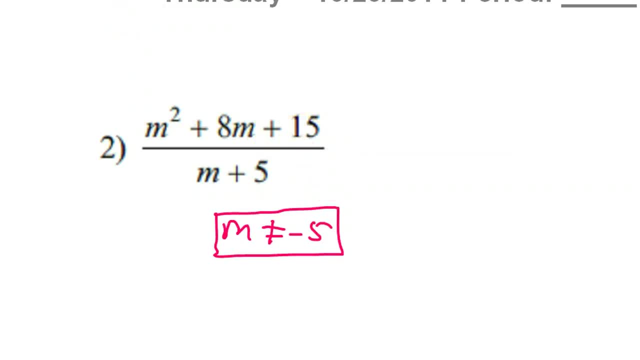 Okay, now let me see if I can factor the numerator or not. So if I try to factor the numerator, there's no common factor. So my only hope is binomial times. binomial m squared is m times m. 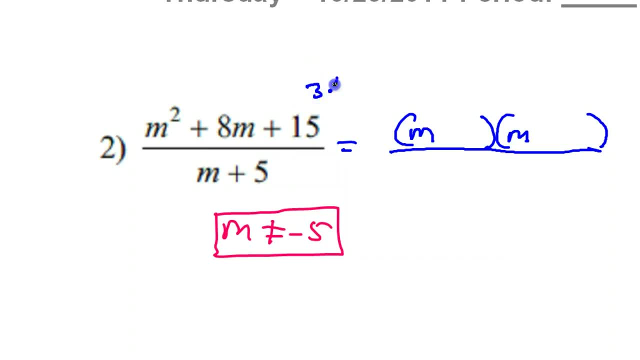 Fifteen could either be three times five or one times fifteen. I'm betting on three times five. Okay, and look, everything is positive. so that would be positive and positive. And yes, inner, I have three m, Outer, I have five m. 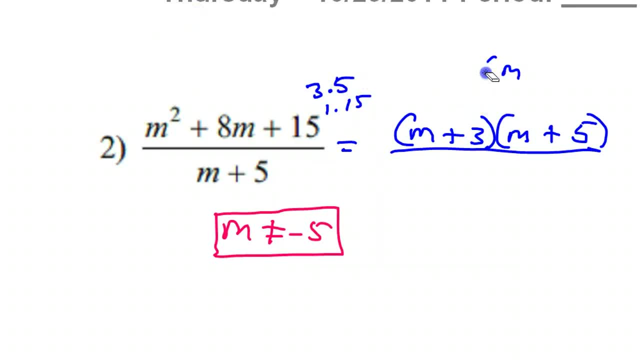 And together that makes eight. so that looks good. So this is how it factors. Now. the denominator is m plus five, which is the same thing I had in the top. So the simplified version. The simplified version is m plus three. 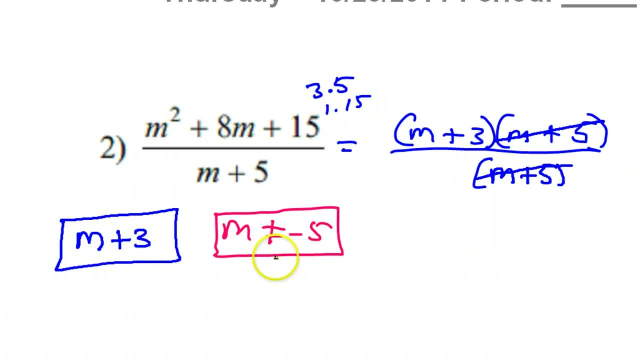 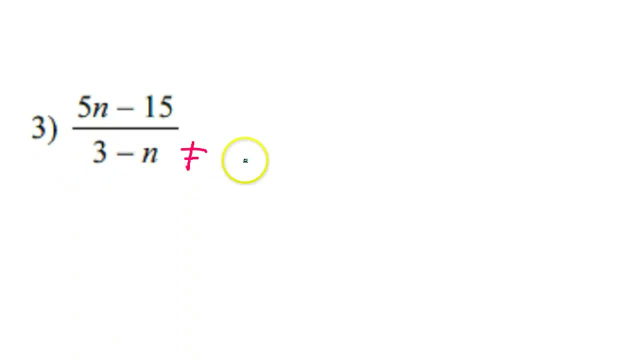 Okay, so there's the simplified answer and the restrictions. All right. looking at number three For the restrictions, I know the denominator cannot equal zero. All right, so subtracting three from both sides, this tells me that negative n cannot equal negative three. 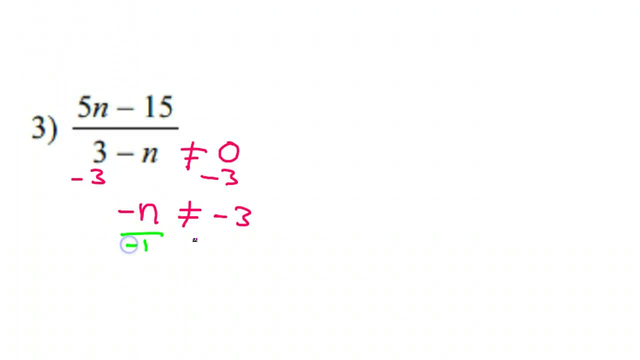 Now, dividing both sides by negative one tells me that n cannot equal positive three. Okay, so this is my restricted value. Okay, now I'm going to go back and find the simplified version of this problem, Okay. Okay, I'm going to factor now. 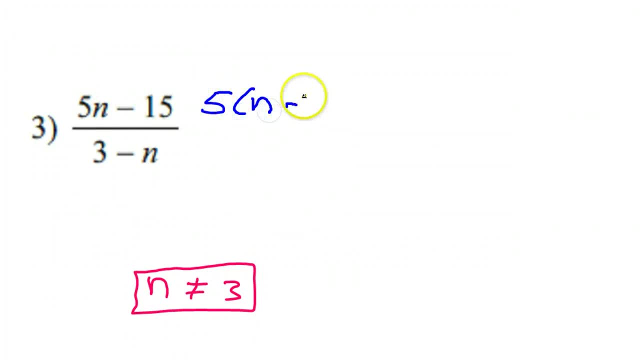 If I factor, that's going to be five times n minus three. Five times three is 15, so it makes sense. Okay, you know what. It's time to talk about something. The meaning to talk to you about something. All right, see how this is backwards. 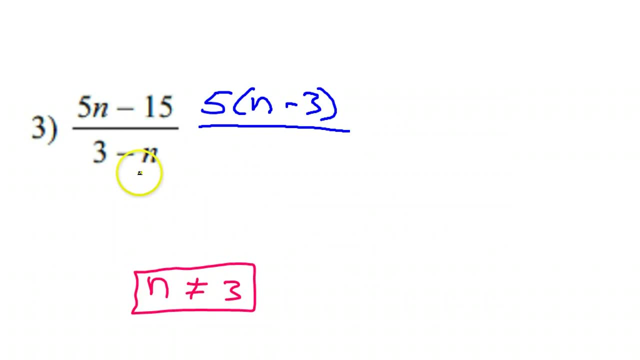 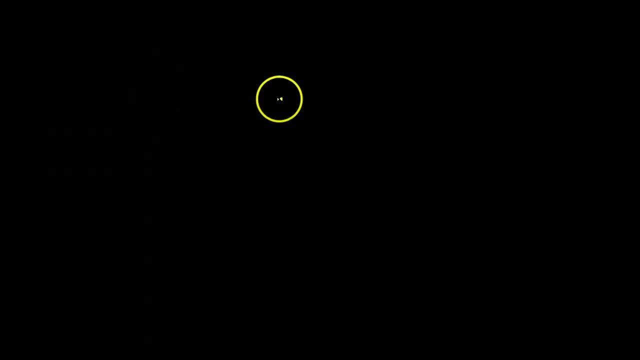 Let's talk about how to fix things that are backwards. Let's have a side lesson. all right, Meet me in the dark room. Okay, Let's have a lesson on backwards binomials. let's say So, for example, say, if I have two minus n. 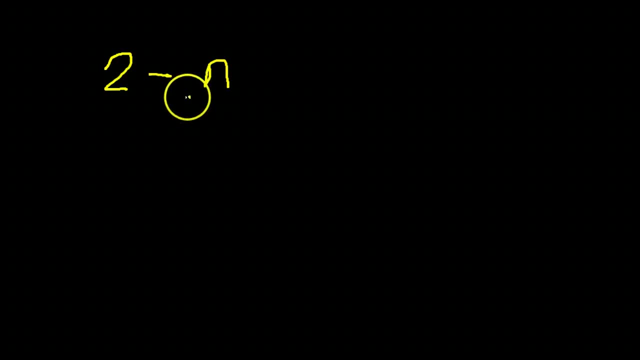 Okay, We know this is backwards. Now, if I switch this around, though, I have to be very careful. all right, This two minus n is sort of like this: It's like I've got a two and I've got a negative n. 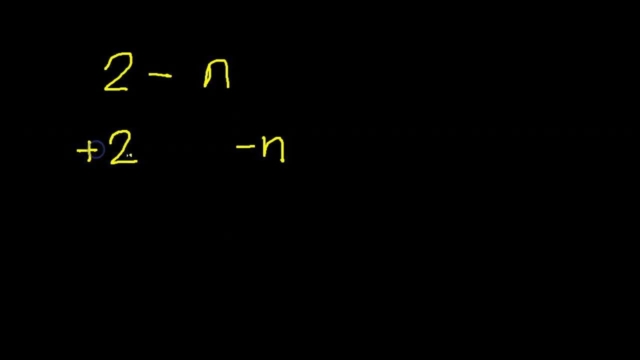 Okay, And in fact you could think of this as a positive two and a negative n. So when we go to switch this around and write it in the proper order, the negative goes with the n, So I will have negative n and then plus two. 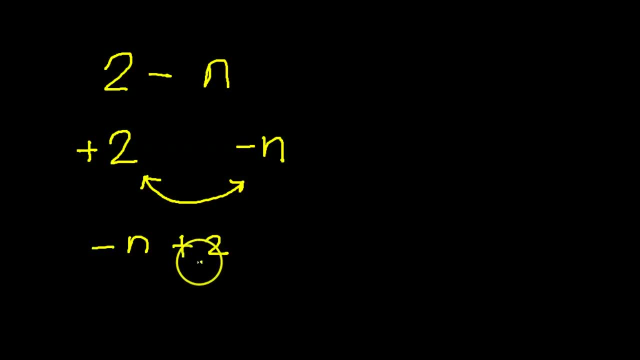 Okay, But when we're talking about factoring and canceling and such, we really don't want the leading coefficient to be negative like this. So what we do is we treat this like a negative one and we factor out that negative one. 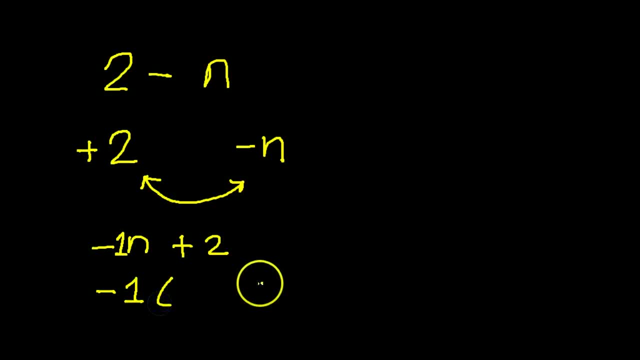 So if I factor out the negative one, you know meaning, put it outside of parentheses- then guess what? Negative one times n would be negative one n Negative one times negative two will be positive two. Okay, So in the end we don't really want to put the one there. 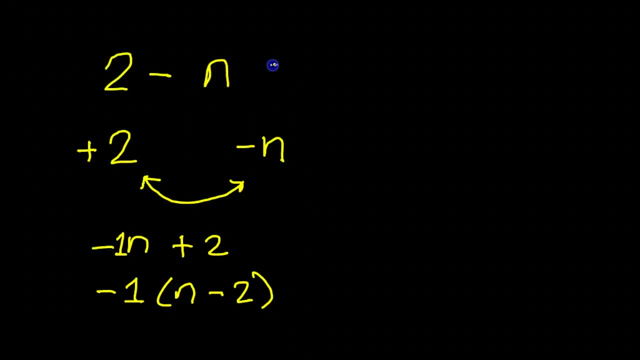 Okay. So in the final analysis, what we have is two minus n is the same thing as negative n minus two. Okay, Okay, Now I don't want to have to go through that process every time. So this little side lesson is to teach you this pattern. 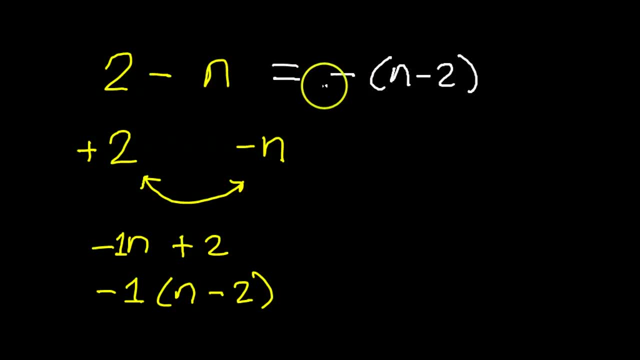 so we can just do it immediately. Two minus n is equal to negative n minus two. Okay, So, in other words, just reversing, you can just swap the two and the n without worrying about the sign. as long as you realize it will be the opposite. 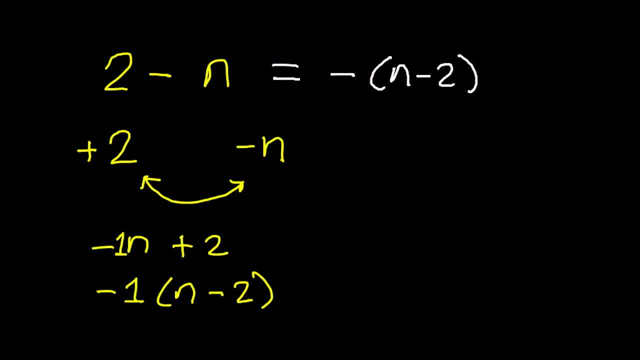 So put a negative sign out front. Okay, Let's practice that skill. Okay. So let's say, if I had five minus p, what would that be equal to Negative p minus five? Okay, What if I had seven minus x? 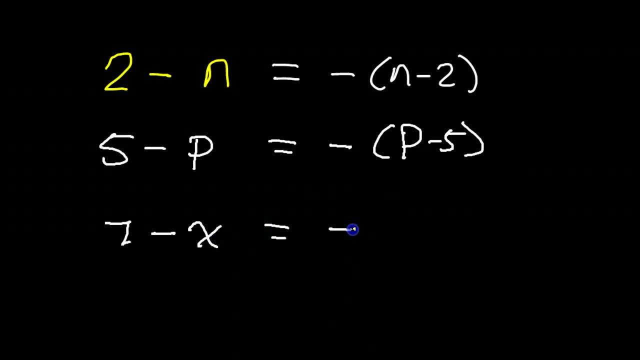 What would that be equal to? That would be negative quantity x minus seven. you see the pattern. um, what if i had x minus y and just for some reason, you know, just do it? um, that would be the same thing as negative y minus x. okay, so that pattern. 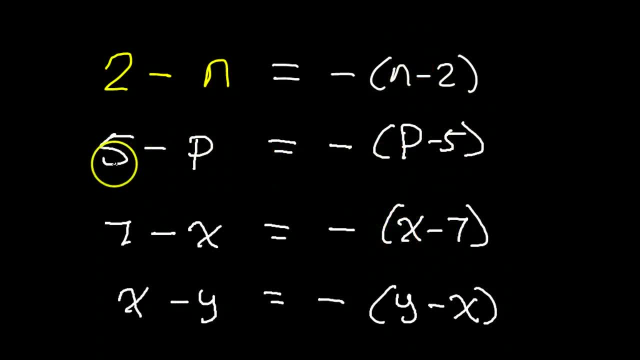 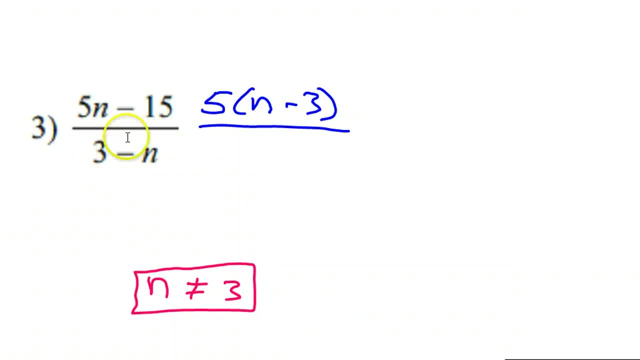 is worth memorizing, so you can just immediately: oh, okay, what it's backwards, write it forwards and put a negative outside the parentheses. okay, um, why am i mentioning that now? well, you tell me three minus n. use the skill i just taught you. what am i going to put? i'm going to put negative. 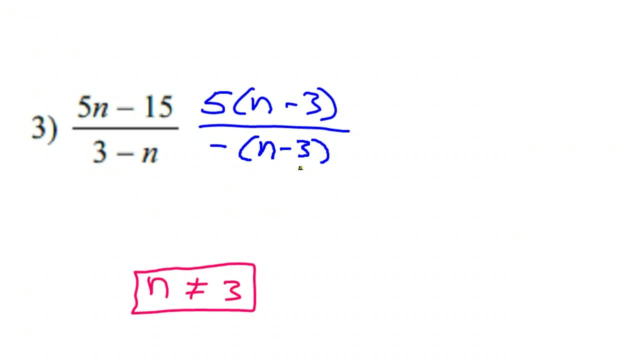 and then just n minus 3.. okay, so now it's easy to see, um, that these will in fact cancel. okay, but you know, i got, i got this negative sign down here floating around. well, it's like a negative one. so, um, it's like i have five divided by negative one, so that's just going to be negative five. 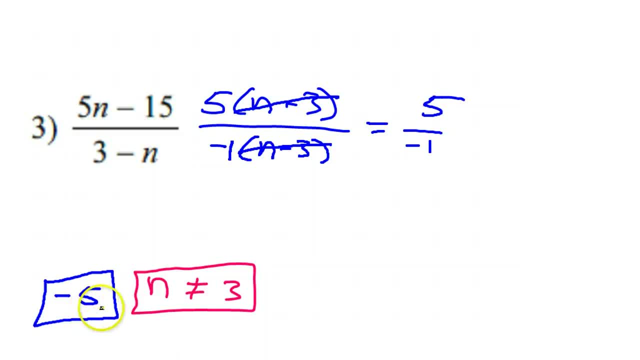 all right. so the simplified answer is negative five. the restricted value is n cannot be three. okay, hope we get to use that skill again at some point in this lesson. i've got to reinforce it. all right, how about this one? so once again, let's find the restricted value. 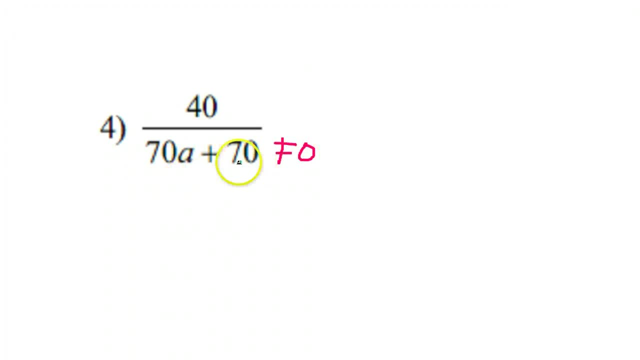 the denominator cannot equal zero. so if i subtract 70 from both sides i get that 70. a cannot equal negative 70. time to divide both sides by 70.. okay, so that is going to give me that a cannot equal negative 1.. so that is my restricted value. 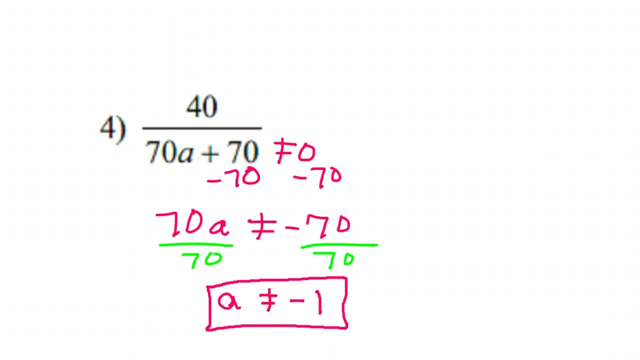 a cannot equal negative 1.. now let's go back and factor okay um factor mode. so i've got 40 over um 70 factors out. so that's going to be a plus 1, right, because 70 times a is 70, a 70 times 1 is 70.. distributive property now um. this will reduce, though, okay. 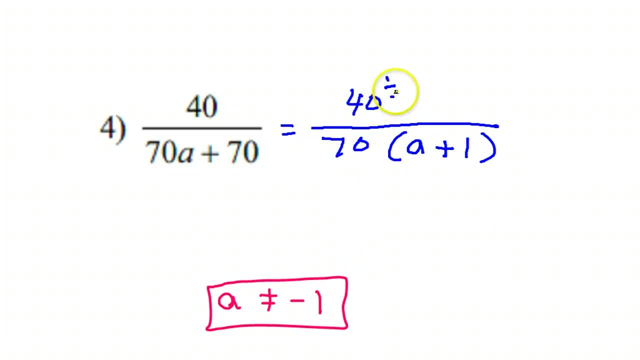 both of these are divisible by 10.. so if i divide by 10, i should use a different color, shouldn't i? um, i could divide both of these by 10.. okay, if i do that, then i'm going to get all right: 40 divided by that's 4. 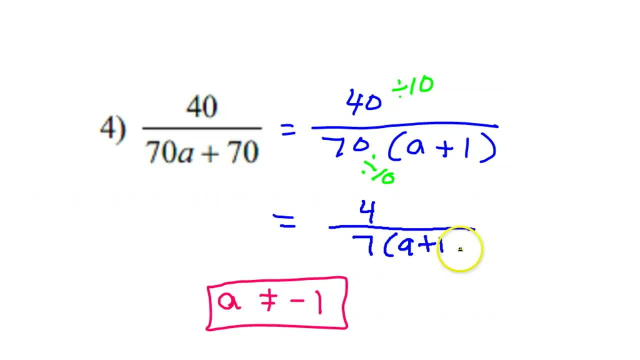 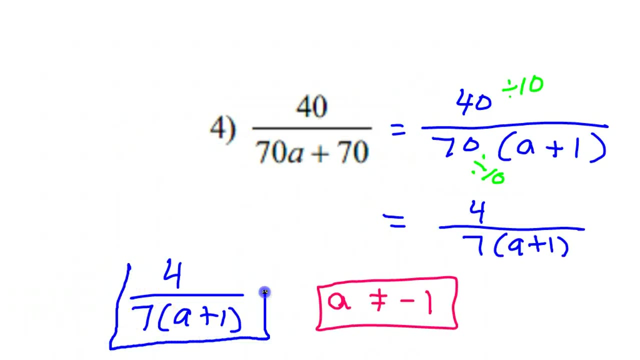 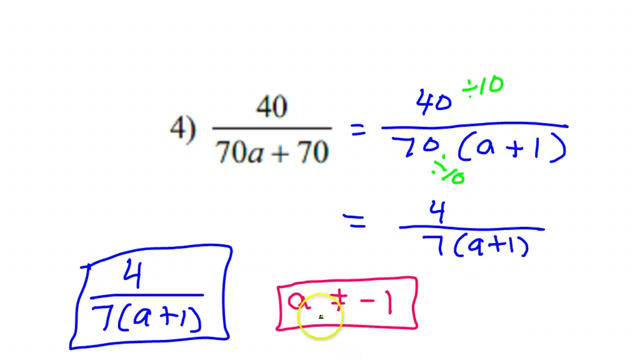 over 7.. and i've still got this a plus 1 going on. okay, so i could write this as my answer. right, i could have 4 over 7 times a plus 1.. okay, um, so here's my simplified answer and my um. restricted value or excluded value. 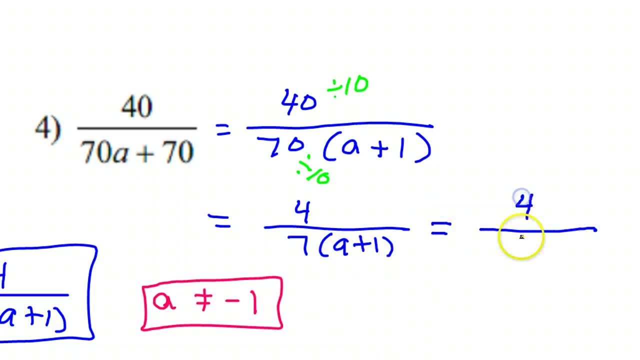 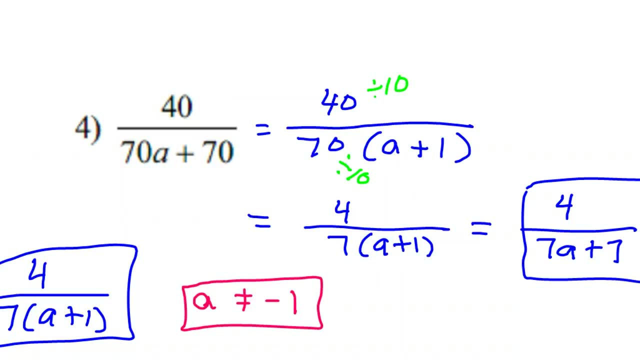 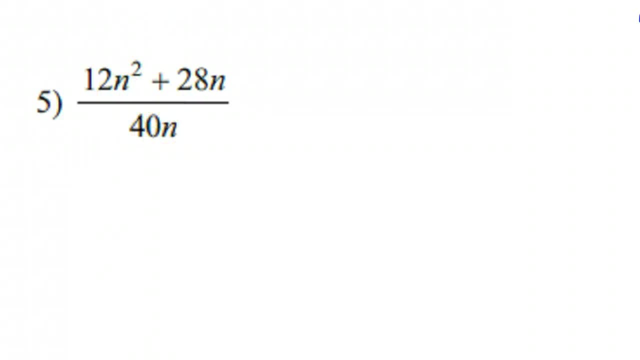 now i could have distributed this and i could have written 4 and then 7 a plus 7.. okay, that's the same thing, so either way. either way, okay, here again, number 5.. If I want to know the restricted values, I will set the denominator not equal to 0, because you can't have that. 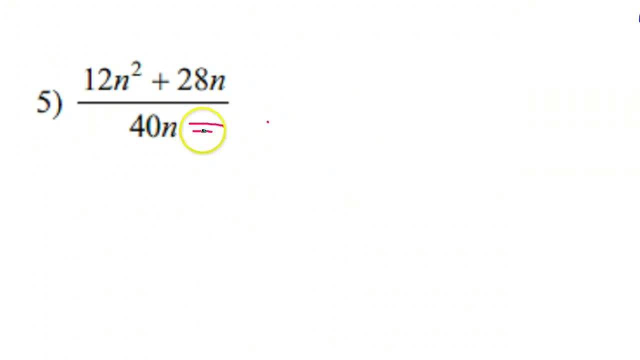 So in this case that means that 40n is not equal to 0. If I divide both sides by 40, then I discover that n cannot equal 0. So that is my restricted value. All right, now for the simplified version. I need to factor. 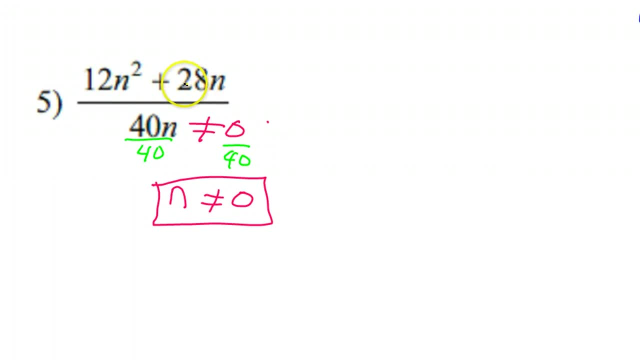 So let's see 12 does not go into 28.. How about, I know 4 goes into 28.. Let's do 4 and see if that's enough. So the GCF here, I think, is 4n. 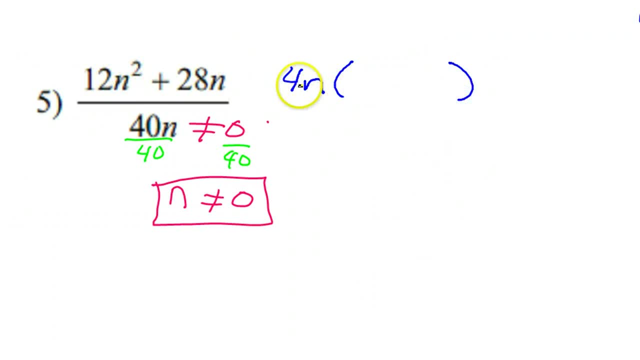 I'll see. I'll see once I see what's left. All right, so that's going to leave 3n plus 7. All right, and there's no more GCF. so I did the right thing And that is over 40n. 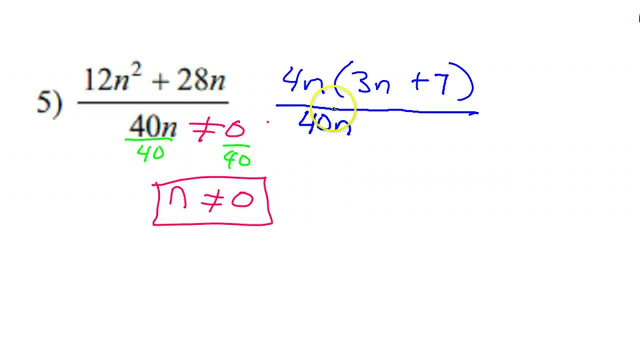 I'm putting it over here on the left because I know I'm about to cancel some stuff out, So I know that these n's will cancel out. All right, this is connected. This is connected by multiplication, so it's okay. All right, so the n's cancel out. 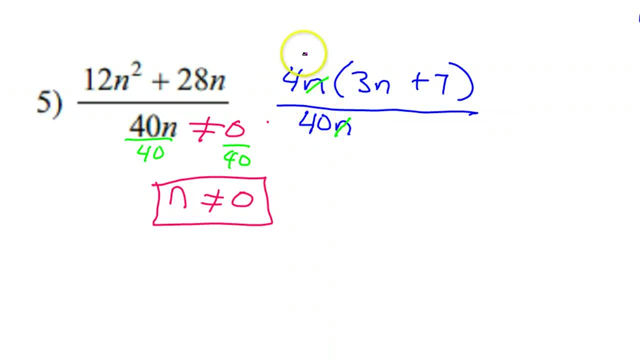 Now the 1 and the- I'm sorry- the 4 and the 40,. these are both divisible by 4.. So that's what I'm doing: I'm dividing these both by 4.. Okay, if I do that, then 4 divided by 4 is 1.. 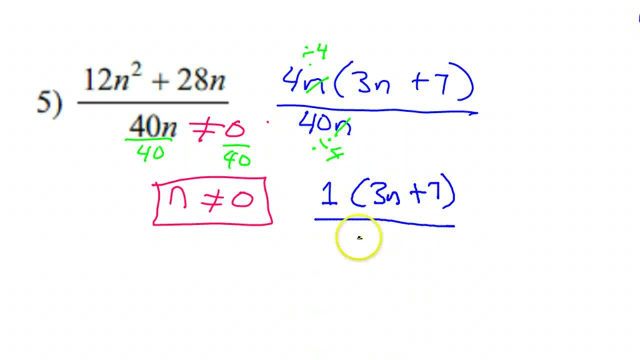 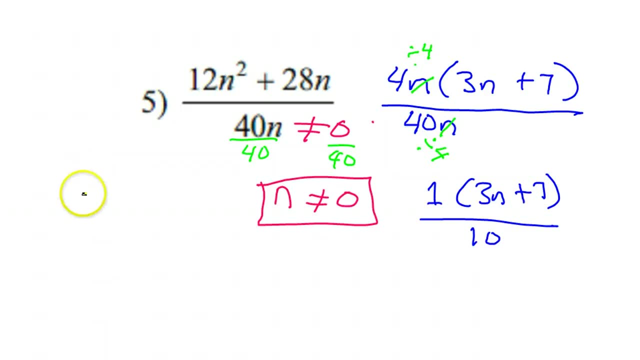 Okay, the n's are gone now. Now, 40 divided by 4 is 10.. Okay, so I really don't need the 1 in the front, though, So I'm just going to have 3n plus 7 over 10.. 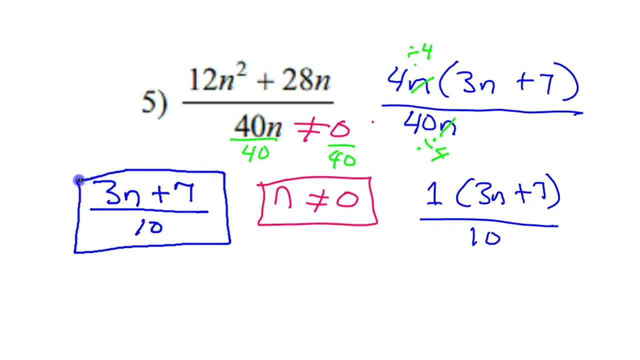 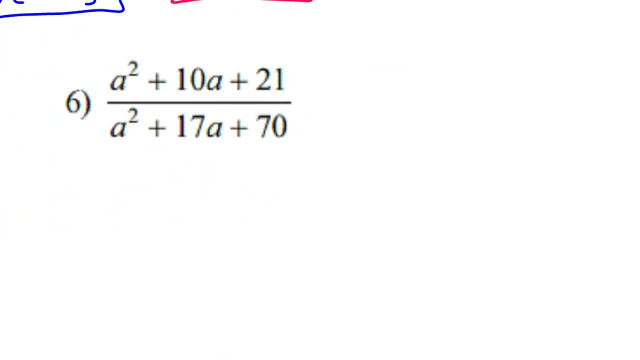 So this is the simplified version And this is the excluded value. So that's number 5.. How about number 6?? All right, I see some factorization In our future here. All right, so in the denominator, a squared is a times a. 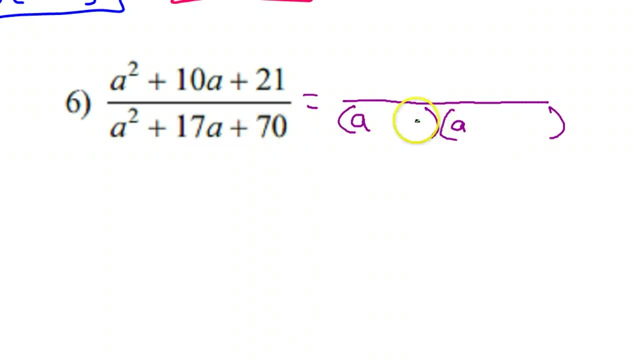 All right, 70. There are other things that can happen, but it's definitely 7 times 10.. All right, which looks promising because of the 17.. You know how we always say: inner plus outer has to give you the middle. 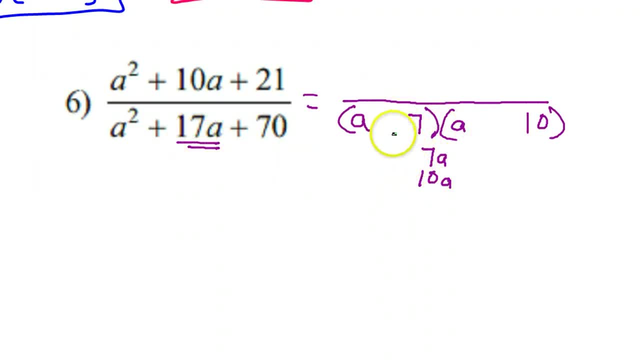 Well, 7 plus 10 does make 17.. So all I need is for everything to be positive, And I am a winner. And positive 7 times positive 10 is positive 70. So that is how you factor the denominator. 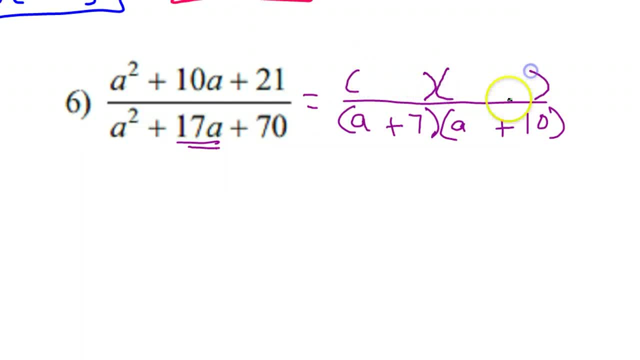 How about the numerator? All right, see how everything is positive. Okay, if everything is positive, that means it's got to be plus and plus. All right, it's no other way. So I'm looking at the 21. The first thing that pops into my head is 3 times 7.. 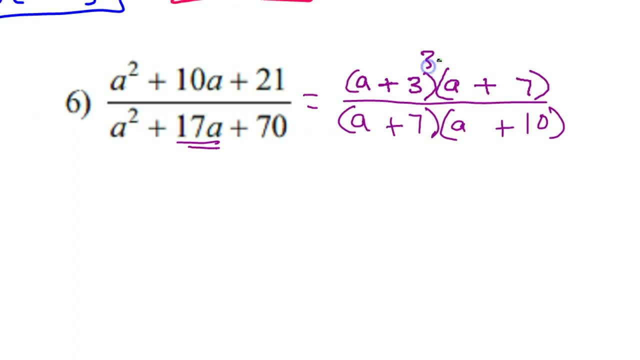 3 times 7 is 21.. And you know, inner plus outer equals middle. 3a plus 7a does make 10a, so we're good. So this is how you factor it. Now let's talk about the restricted values. 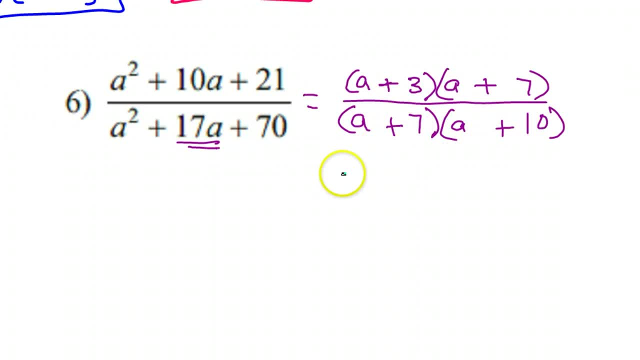 The denominator cannot equal 0. That means neither one of these factors can equal 0.. a plus 7 cannot equal 0.. a plus 10 cannot equal 0.. Subtracting 7 from both sides tells me that a cannot equal negative 7.. 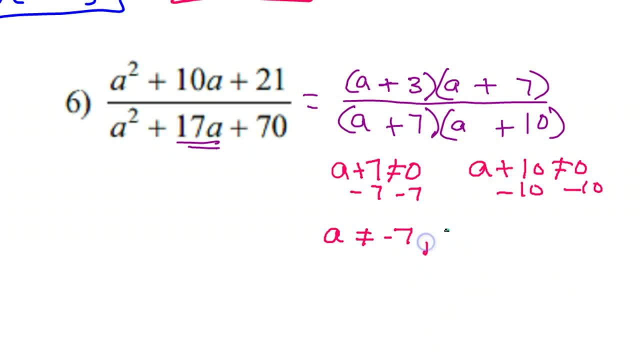 Okay, subtracting 10 from both sides tells me that a cannot equal negative 10.. So these are my restricted values. Okay, now let's talk about the simplified form of this. Well, all that's left to do is cancel out the a plus 7s, which are the same factor. 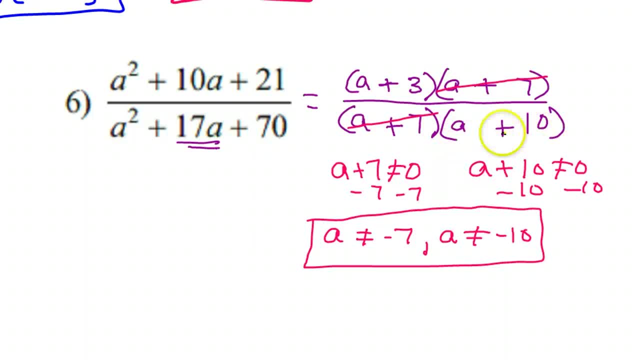 And that is going to leave a plus 3 over a plus 10.. So I've got a plus 3 over a plus 10.. And that is the final answer. Please do not think you can cancel out these a's, okay. 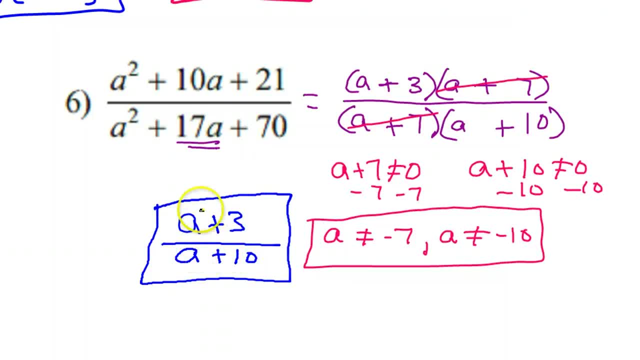 When things are connected by addition or subtraction, you can't cancel them out. Okay, that doesn't make any sense. So that's it: a plus 3 over a plus 10.. And these are the restricted values, the excluded values. 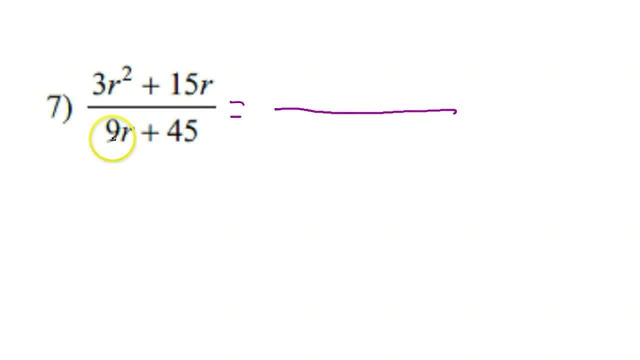 Let us factor: 9 is the GCF here, So that would be 9 times r plus 5.. Here the GCF is 3r And that's going to leave behind r plus 5.. Now, as far as the restricted values, please understand that only r plus 5 has to be worried about. 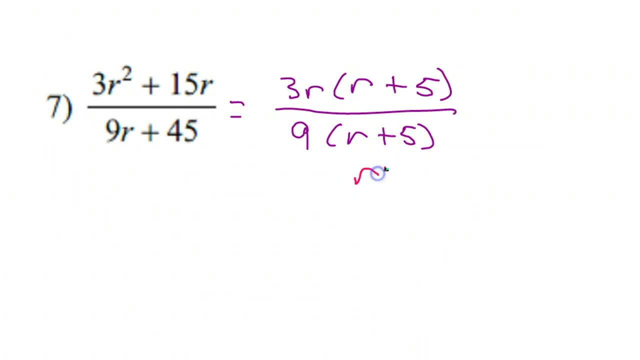 Okay, r plus 5 cannot equal 0.. All right, 9 is 9 is already not 0,, so I don't have to worry about that. If 9 times something is in the denominator, the only thing we have to worry about is making. 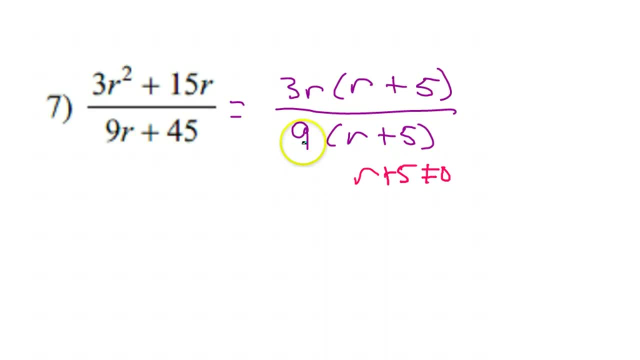 sure that r plus 5 is not 0.. 9 is not going to turn into a 0, so ignore that. Meanwhile, over here, subtracting 5 from both sides, r cannot be negative 5.. So that is my restricted value. 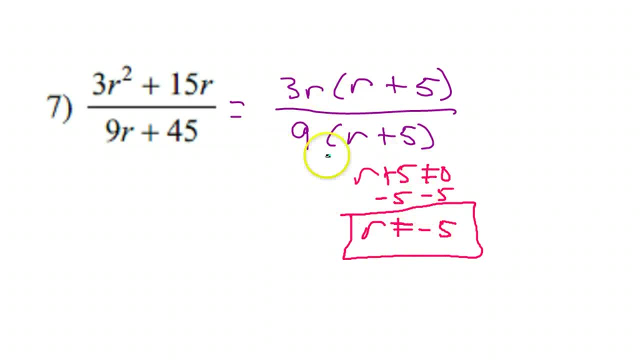 Just one restriction. Okay, Now, as far as the simplified form just cross out, these r plus 5s And we need to reduce these as well. All right, Both of these are divisible by 3. So you've got to do it. 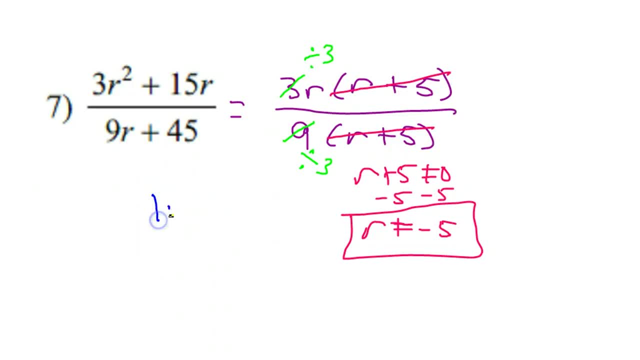 Okay, 3 divided by 3 is 1.. So that's like 1.. 1r over 9 divided by 9, divided by 3 is 3.. So it's like 1r over 3.. But do we really need the 1?? 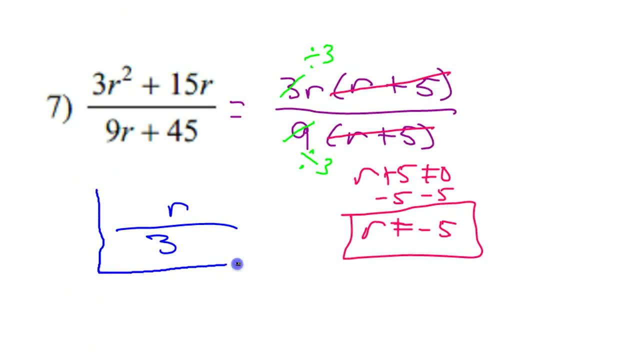 No, So it's really just r over 3.. So there it is: r over 3.. r cannot equal negative 5.. By the way, do you have a pen or a pencil in your hand? No, So you don't need a pen or a pencil in your hand. 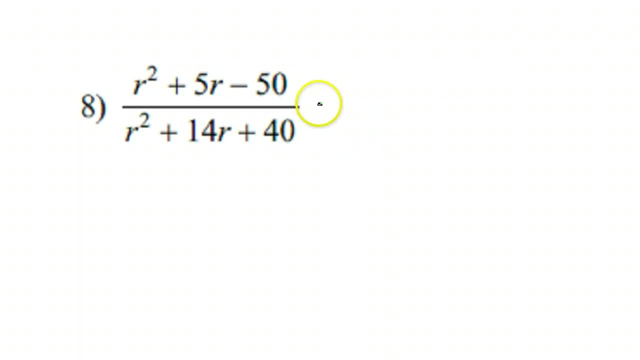 Well, if you do put it down, Shame on you. Don't? I talk to you about this every day. If you just copy off of me, you're not going to learn anything. All right, Put the pencil down. Try to do the problem by yourself first. 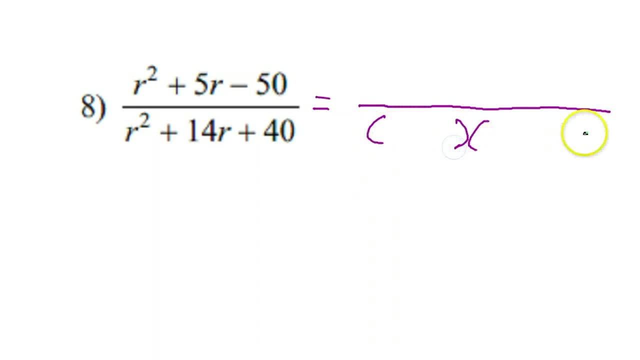 If you're still getting it wrong, watch the video and learn how to do it, But then go back and do it by yourself, Factoring the denominator I'm thinking: well, I'm going to do this, I'm going to do this. 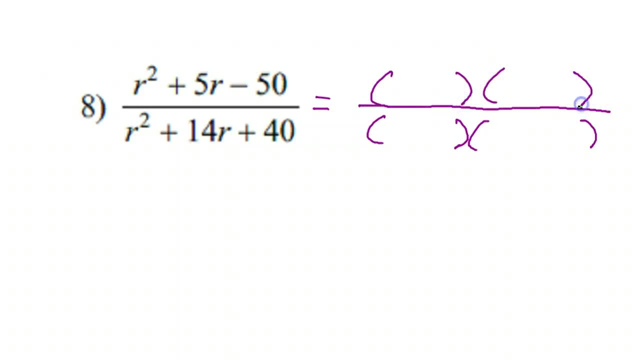 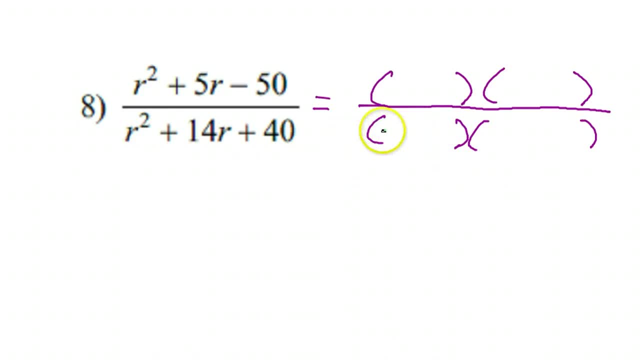 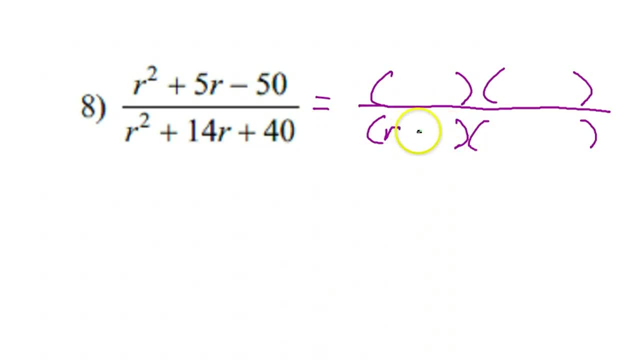 Factoring the denominator. I'm thinking r plus 4 times r plus 10.. Right, Four plus- I'm sorry- Four times 10 is 40. Okay, And that gives us inner 4r, outer 10r. 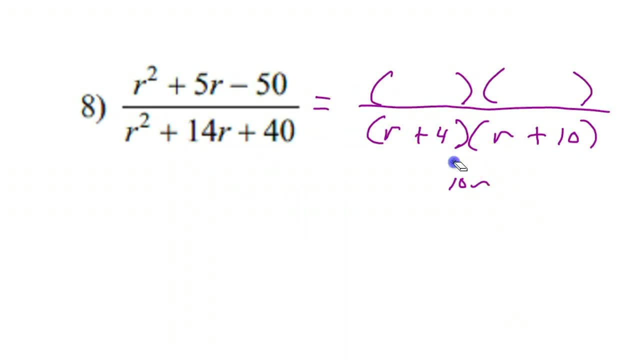 Well, that makes 14.. So that's why I like that. Okay. Okay, R squared in the numerator here, R squared is R times R, Now 50,. okay is 5 times 10.. Okay, so I'm going to need a positive 10 and a negative 5 to make a positive 5R. 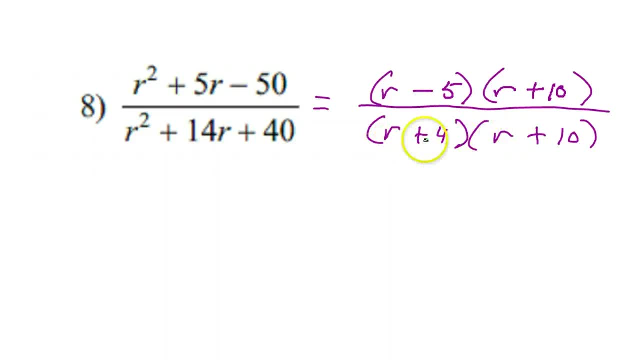 Okay, so as far as the restrictions, both of these are going to give me an excluded value. Okay, because R plus 4 cannot equal 0, and R plus 10 cannot equal 0. Subtracting 4 from both sides, R cannot equal negative 4.. 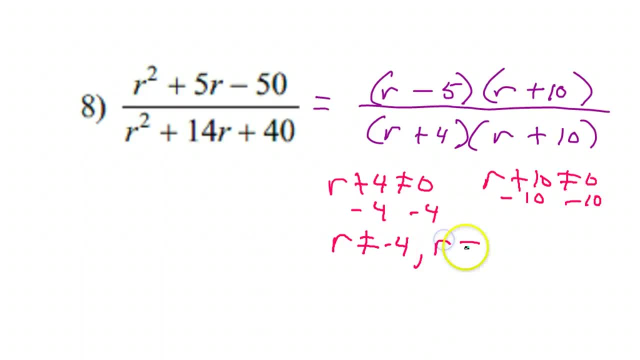 Subtracting 10 from both sides, R cannot equal negative 10.. So those are the restricted values. Once I calculate them, I'm going to need a positive 10.. If I cancel out the R plus 10s, that's going to leave me with R minus 5 over R plus 4.. 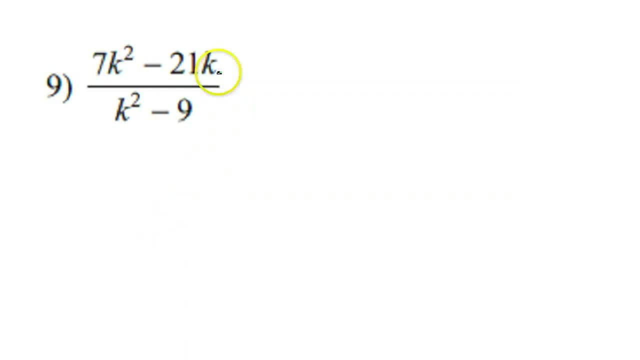 Okay, that's it for number 8.. All right, we are down to the last couple problems, which is good, because I'm starting to lose my voice. This is the difference of two squares, So this is going to factor as K plus 3.. 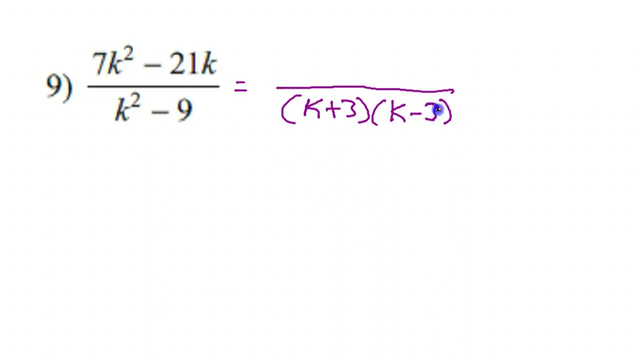 Times K minus 3.. Okay, meanwhile, the numerator has a GCF, a common factor of 7K. Okay, that's going to leave behind K minus 3.. Both of these factors will give me a restricted value, Because K plus 3 cannot equal 0.. 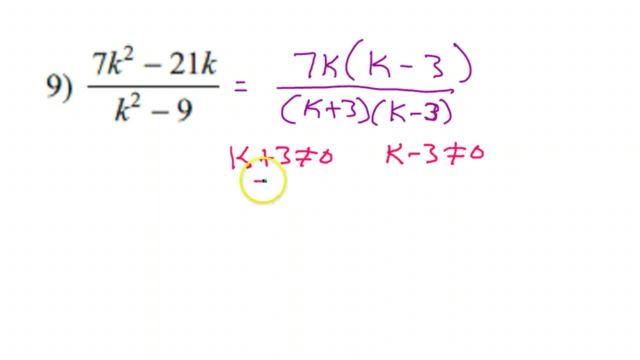 And K minus 3.. Subtracting 3 from both sides gives me K cannot equal negative 3.. Ah, Adding 3 to both sides gives me K cannot equal positive 3.. So these are my restrictions. Okay, that's it. 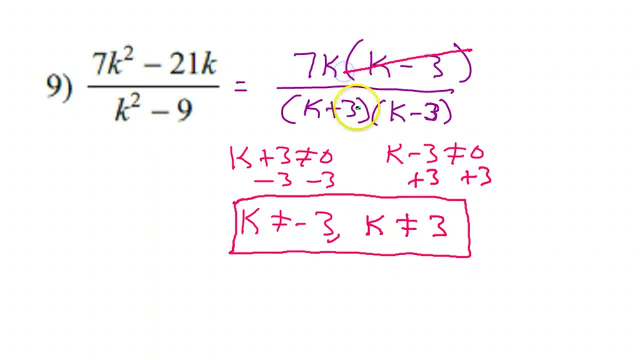 Now, as far as the simplification of this, I'm going to need to do a little bit more. As far as the simplified version, the K plus 3s cancel out. So that's going to leave me with 7K over K minus 3.. 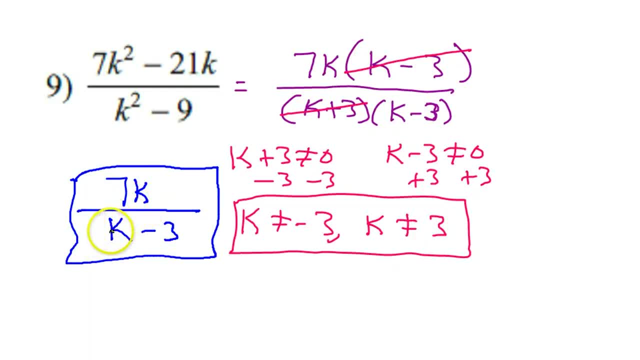 All right. notice that you cannot cancel out these Ks because this is connected by subtraction. All right, if this were 3K instead, I could do the same thing. Instead. I could do the same thing. Instead, I could cancel them. 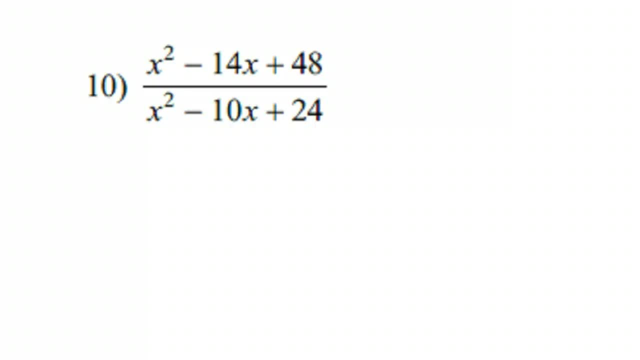 So that's number 9.. All right, this is the last problem. Okay, let's factor X squared X times X 24.. It could be 6 times 4, or 4 times 6.. Oh well, that's the same thing. 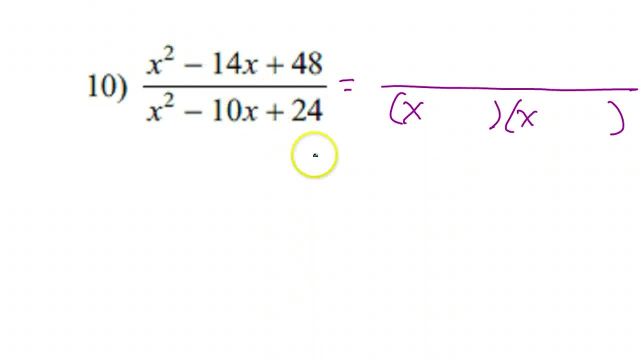 It could be 4 times 6, or 2 times 12, or 1 times 24.. Oh, I left out the 3.. Or 3 times 8.. I knew I was missing something. Anyway, based on the 10, I'm betting on, well it could be. either one of these could make a 10.. 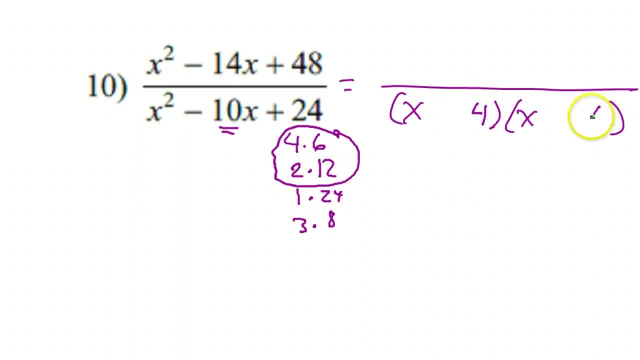 Okay, let's try the 4 and 6 first. If I do the 4 and 6, because I'm thinking, oh look, there's a 10. Inner plus outer has to give me the middle Inner, I have 4X. 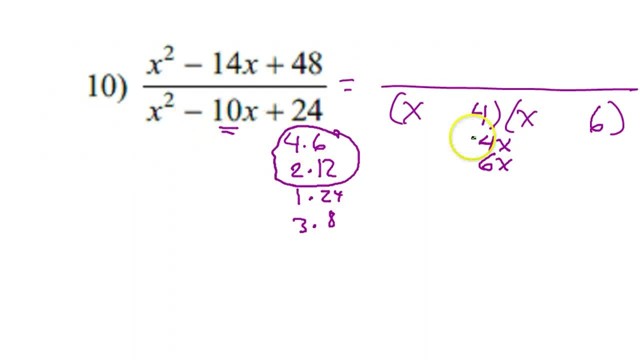 Outer, I have 6X. If I want to get a negative 10, both of these have to be negative, So I would make these both negative. Will that give me a positive 24?? Yes, because a negative times a negative is a positive. 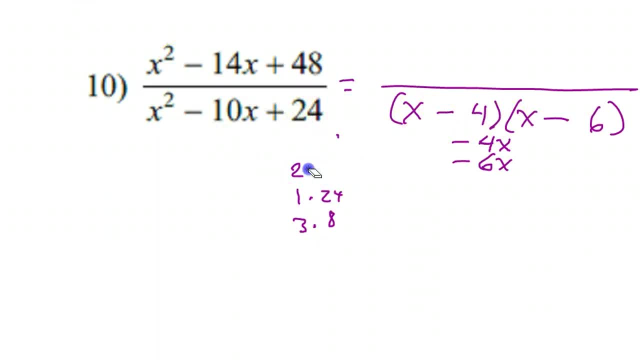 So that's how you factor it. Erase all this stuff now. Okay, now the numerator. Okay, X squared, It's clearly X times X. When I look at 48, the first thing that pops into my head is 6 times 8 is 48.. 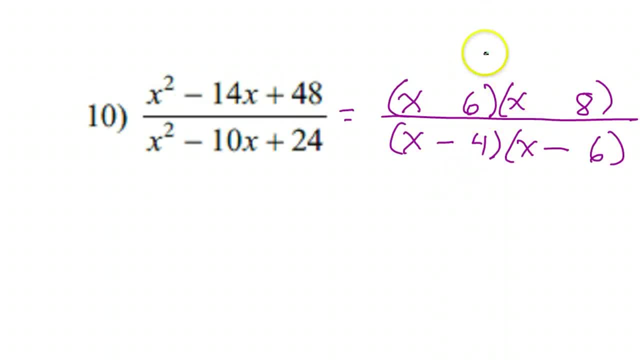 Okay, and inner I have 6X, Outer I have 8X. Let's see, is there a way I can get negative 14 if I pick the signs right? You bet your sweet bippy If they are both negative.